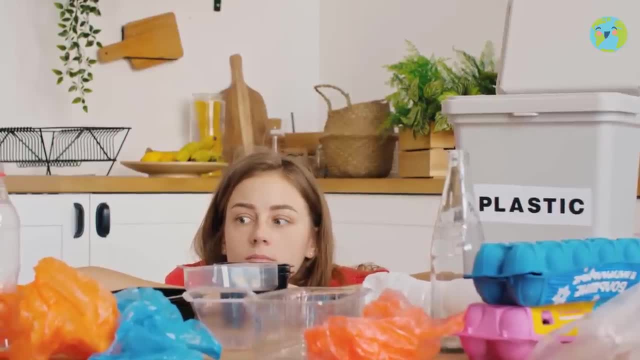 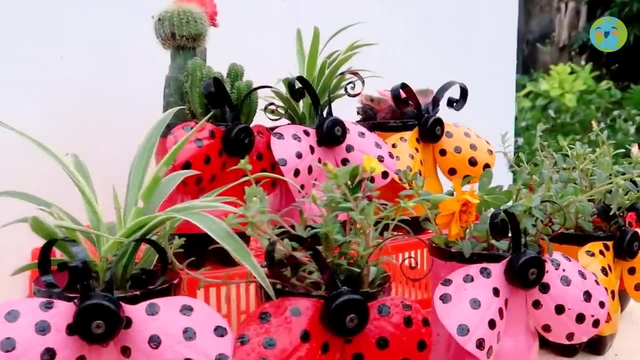 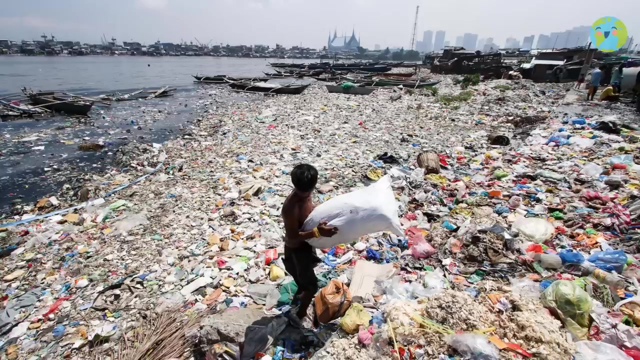 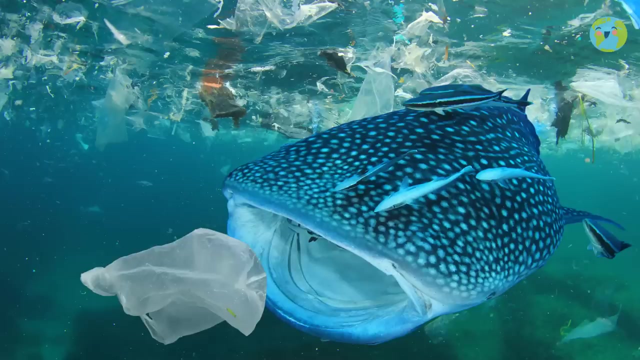 Just buy what you're used to. Here. imagination and creativity are super important. You can, for example, make a nice flowerpot with the empty soap bottle, so it won't have to go the trash. Well, did you know That every year, huge islands of garbage are created in the oceans? that cause the death of millions of marine animals? 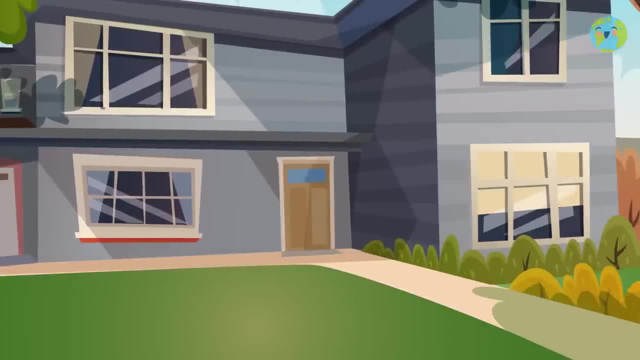 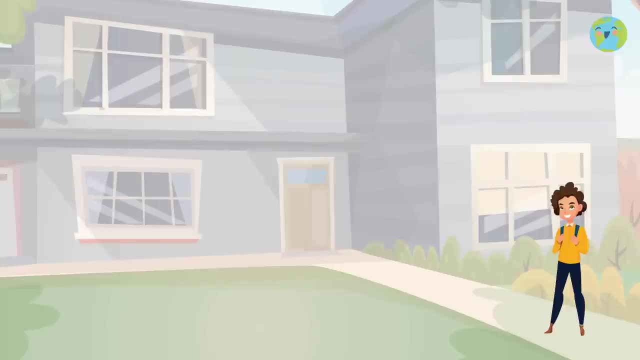 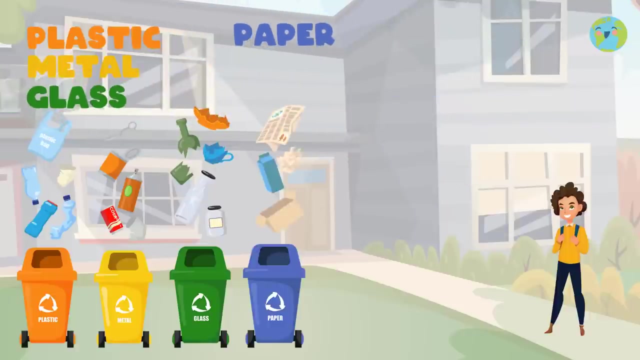 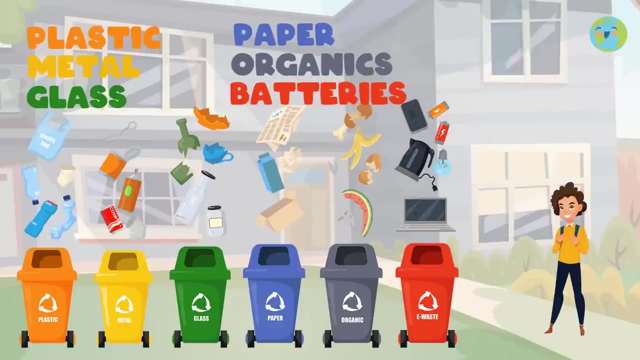 Oh, The good thing is that you can help a lot from home if you start with the habit of recycling. The idea, my friends, is to separate plastic, metal, glass, paper, organics and batteries in the corresponding garbage cans according to their color. 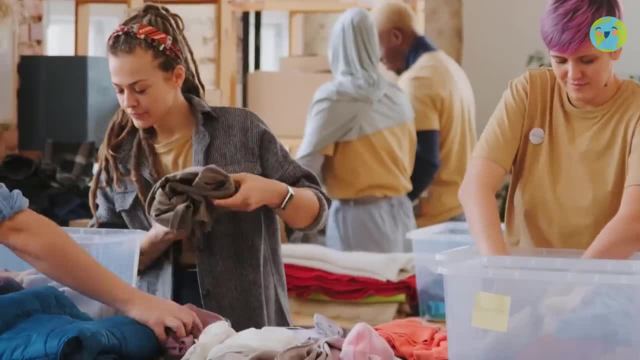 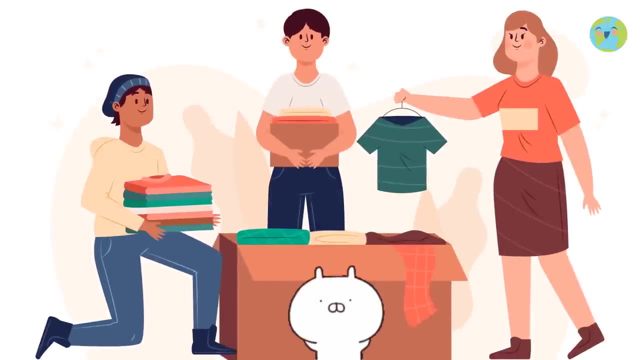 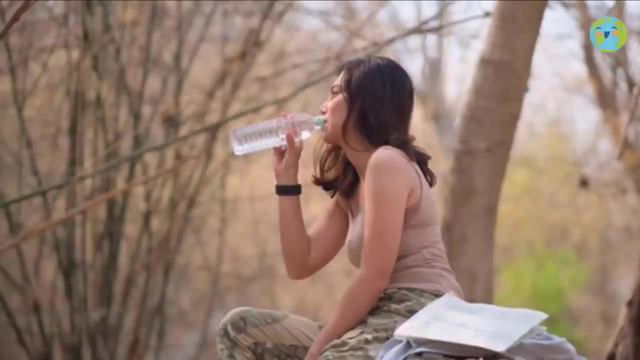 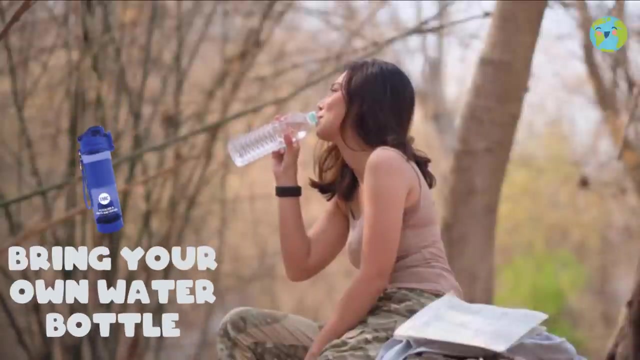 Reuse. A great example is to donate clothes that are in good condition but you no longer use, so another child can reuse them and you also do a good deed Reduce. A great way to use fewer products that pollute a lot like plastic is to make sure you bring your own water bottle every time you go out. 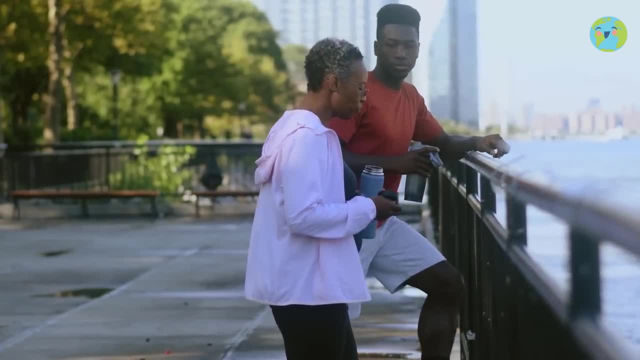 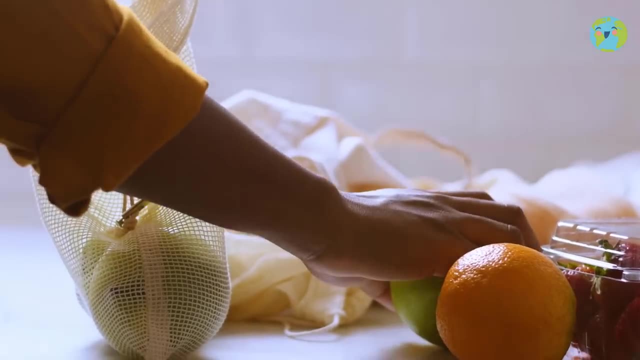 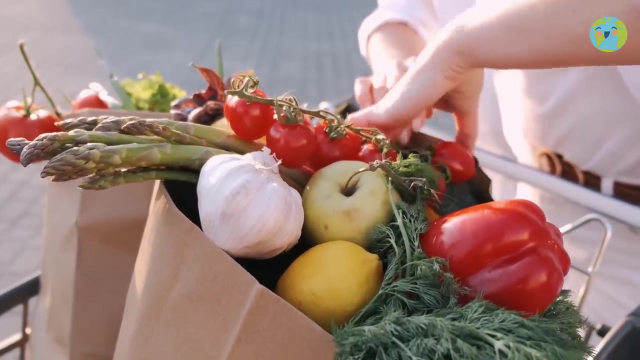 so you don't have to buy a plastic. You can also buy a plastic one on the street. Take your own bags with you. As long as you remember, pack a- preferably cloth- bag in your backpack so when you go to the supermarket or shopping with your parents, they don't need to ask for plastic bags. 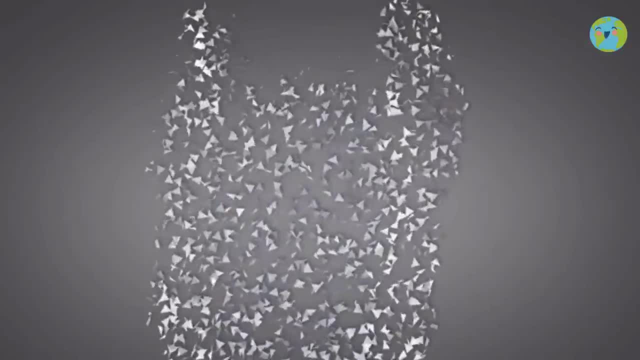 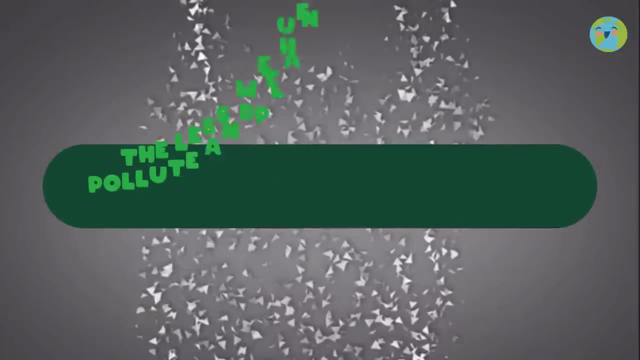 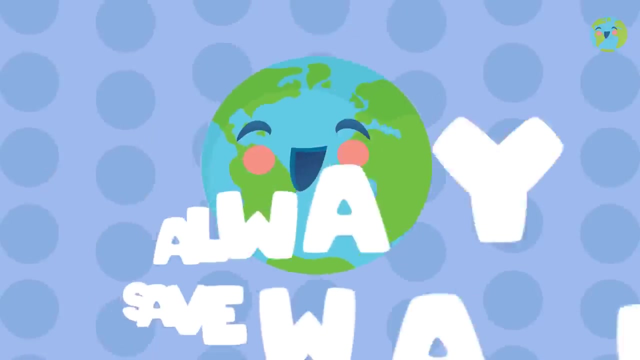 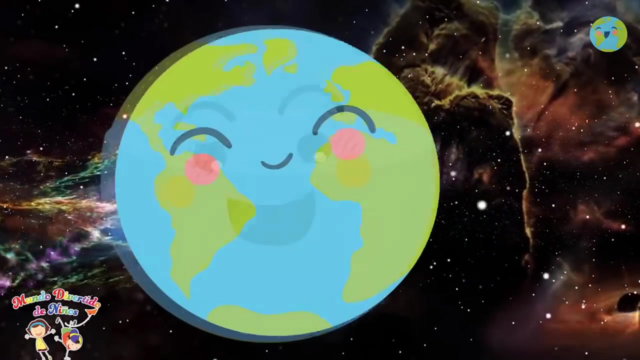 What happens, guys, is that a single plastic bag takes more than 150 years to decompose. so the less we use, the less we pollute and the better for the planet. Always save water. In my other video about water and its care, I tell you the importance of this precious liquid of life and how you can help take care of it.